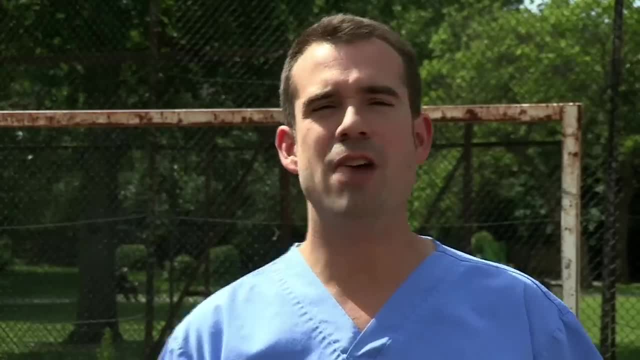 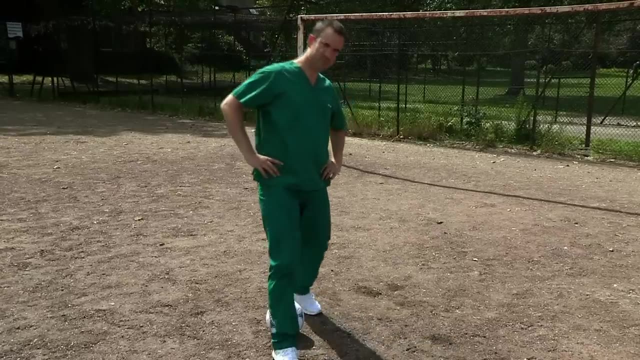 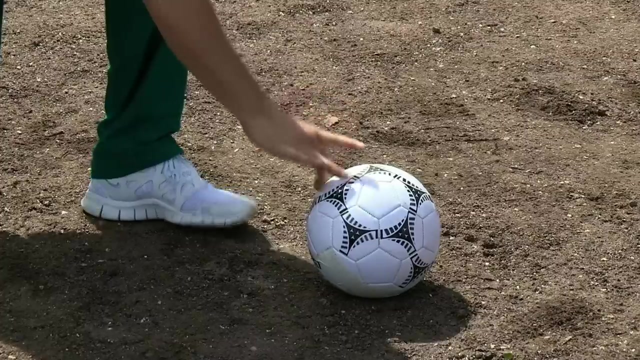 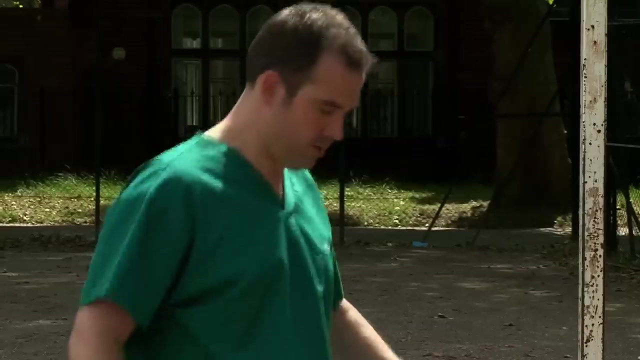 Nothing beats a spot of football in the park: Fresh air, aerobic exercise and, of course, the chance to show off those silky football skills like the step-over or the cry of turn or the rainbow flick. But football can also be dangerous. You could turn sharply and twist an ankle. I don't think so, Chris. 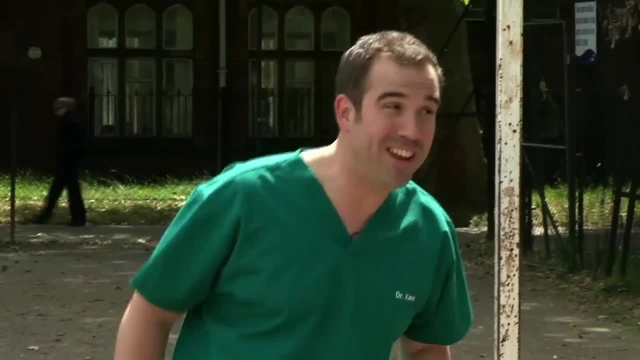 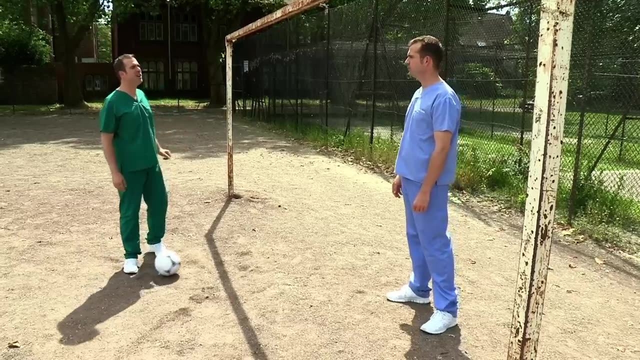 Well, well, you could injure yourself if someone tackled you- Very unlikely in my case. You could break your fifth metatarsal kicking the ball too hard. My metatarsals are as hard as toughened steel, All right, well, look, just be. 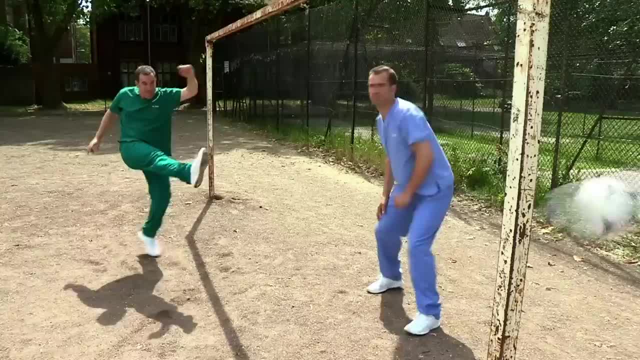 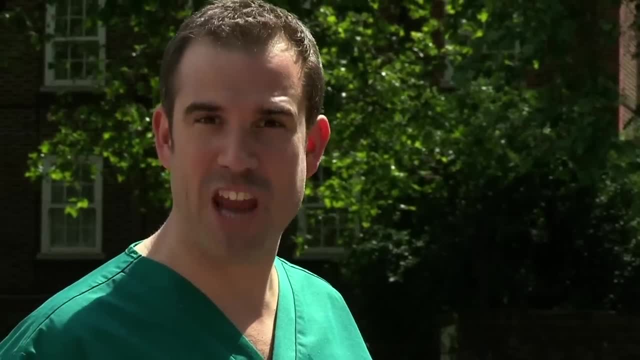 careful when we're playing. Now, Zandi on me head son. That manoeuvre's known as the Chris Clonk, but it's also an injury alert. Wow, Chris is very good at pretending to be knocked out, isn't he? 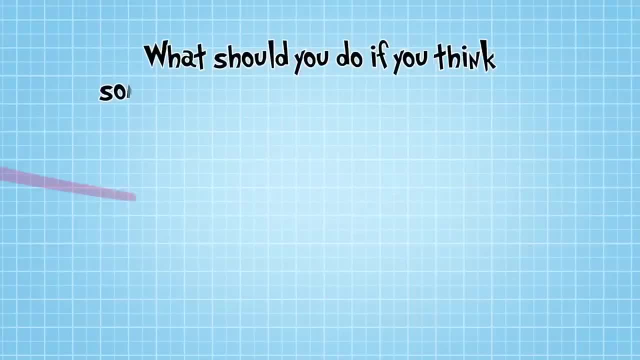 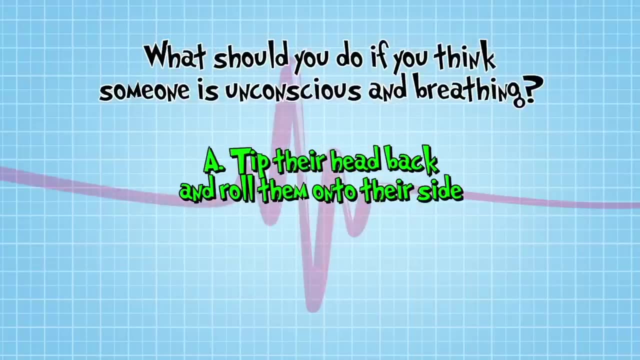 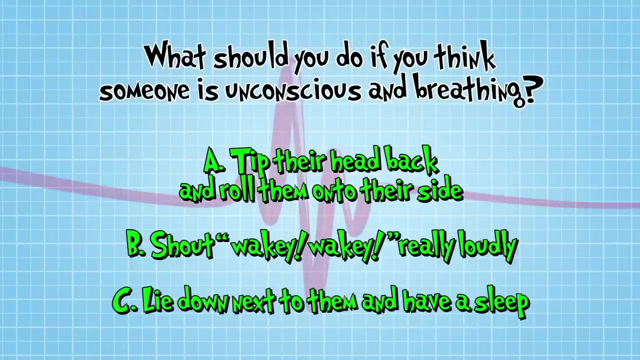 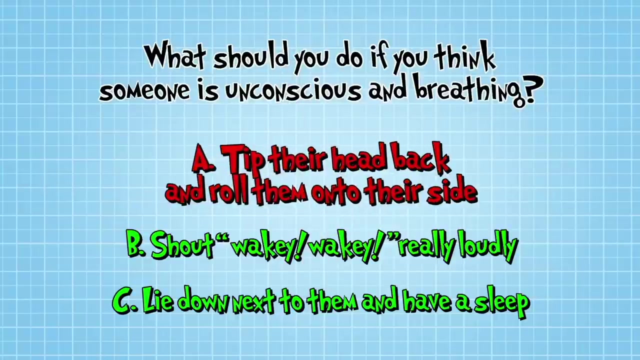 So what should you do if you think someone is unconscious and breathing? Tip their head back, check they are breathing and roll them onto their side, Shout wakey, wakey, really loudly, Or lie down next to them and have a sleep enjoying the peace and quiet. The answer is A: Tip their head back, check their. 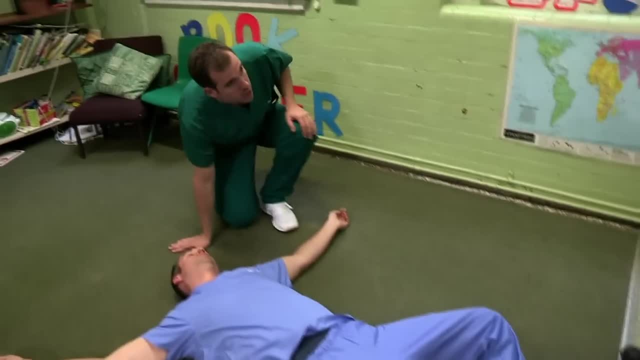 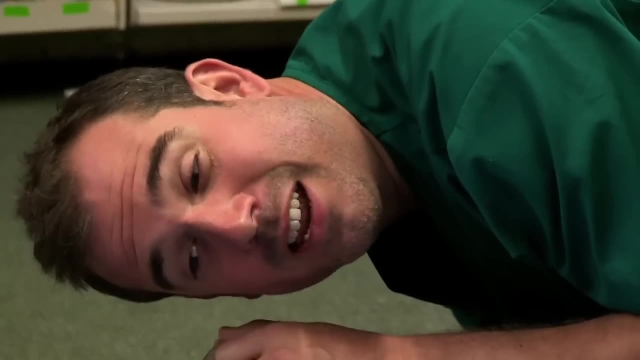 breathing and roll them onto their side. First thing we want to do is check if he's breathing. We tilt his head back a little bit so his airways open and then have a listen. I can feel his breath on my ear and I can see his chest moving, so 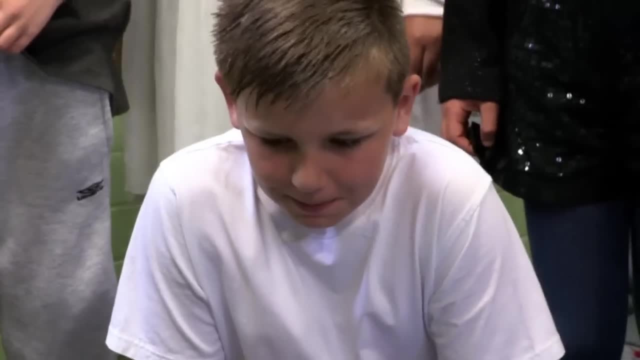 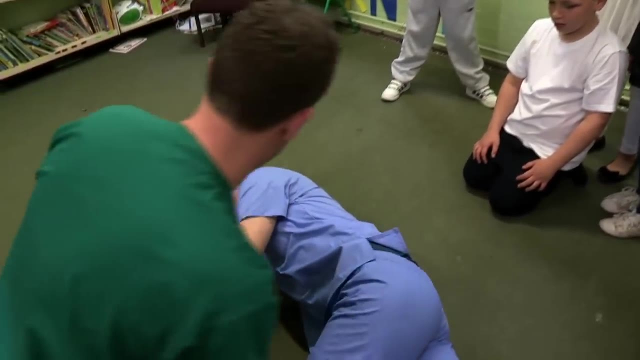 we definitely know he's breathing. So now we need to roll him onto his side So we get his leg up here, get his arm over here, and then we can pull him this way, And then we can use this hand to support his head. And now, if he's sick, it goes on. 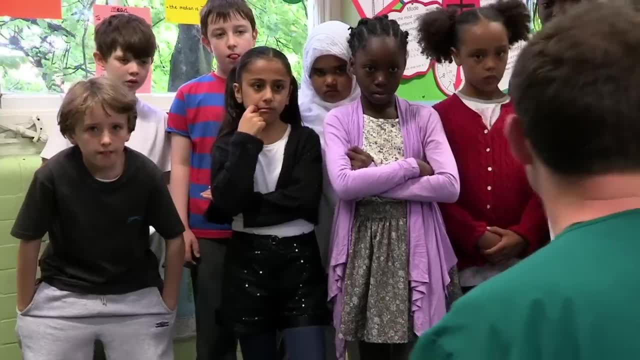 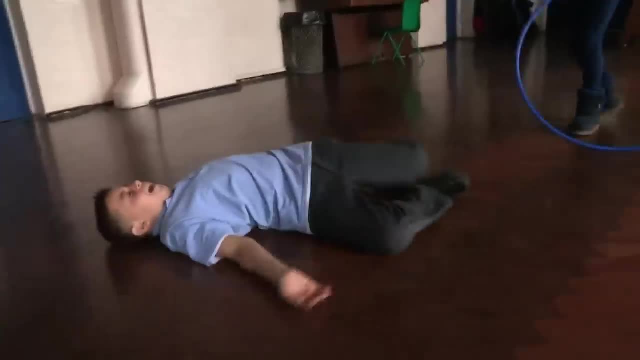 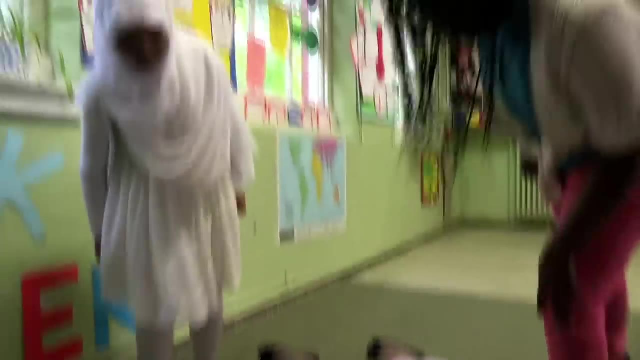 the ground. his tongue is gonna fall forward, so it won't stop him breathing and we can go and get help because he's nice and safe. Let's give him a go. Me Remember: never do this on your own, unless it is an emergency. It's always best to find an adult.